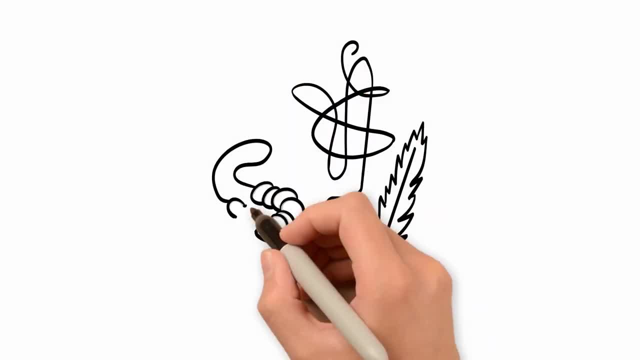 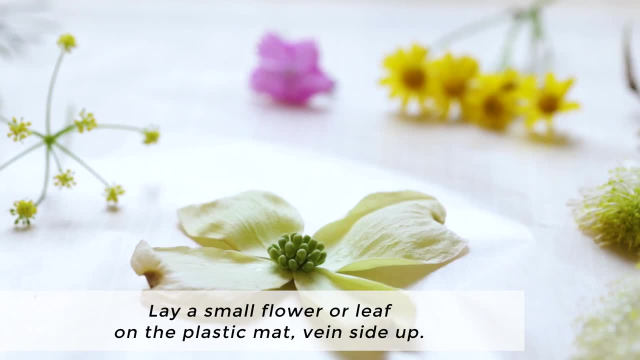 other side of your work surface. This will protect your work surface, but also will keep the air dry clay from clinging to another surface. Next, lay a small leaf or flower on the wax paper, and this works especially well if you do it vein-side up. 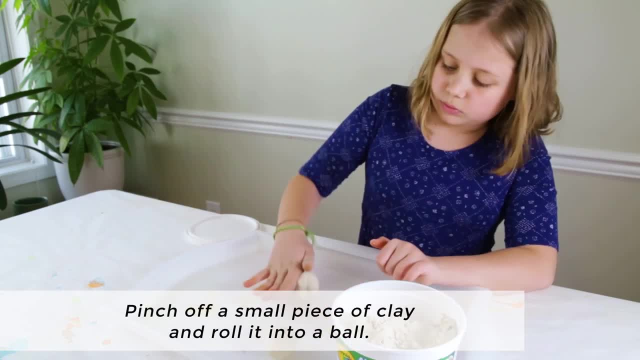 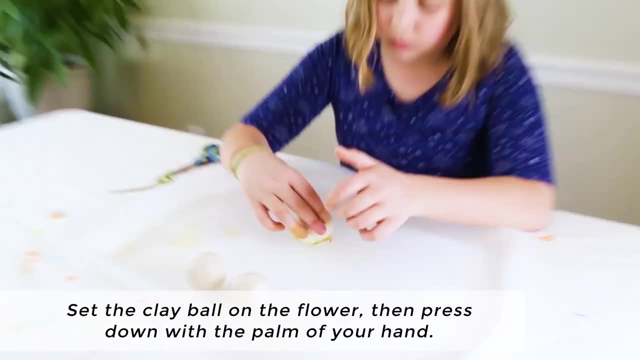 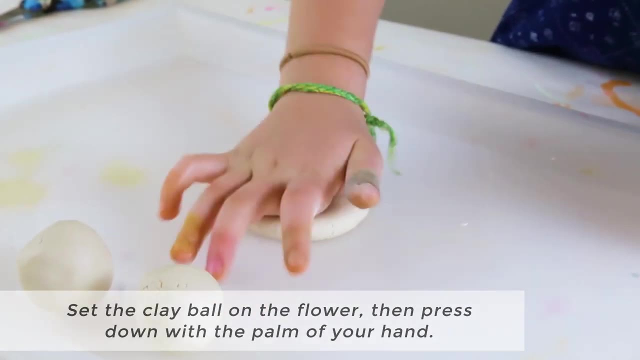 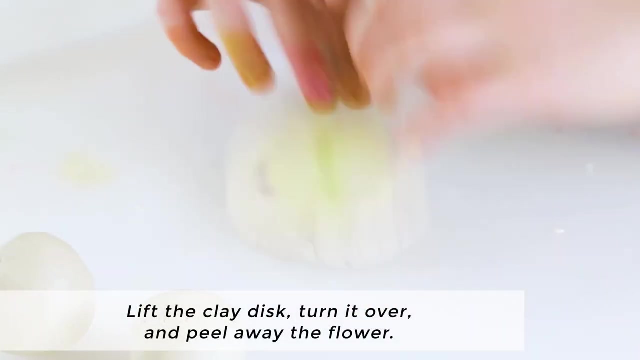 Then pinch off a small piece of clay- about a tablespoon or two- and roll it into a ball between your hands. Then set the clay ball on the leaf and press down with the palm of your hand to flatten it. Once you have flattened the clay, you can take the object off the work surface and push it. 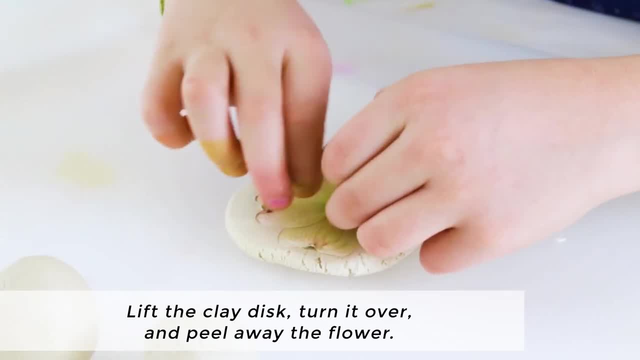 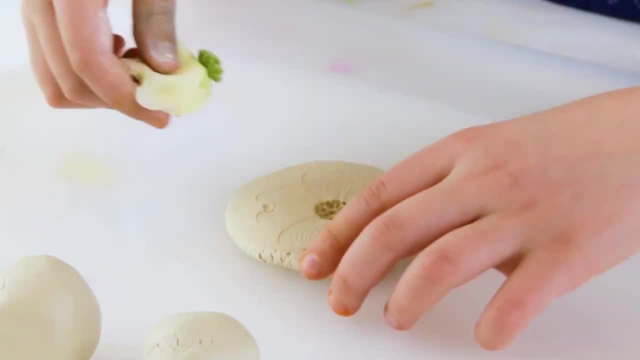 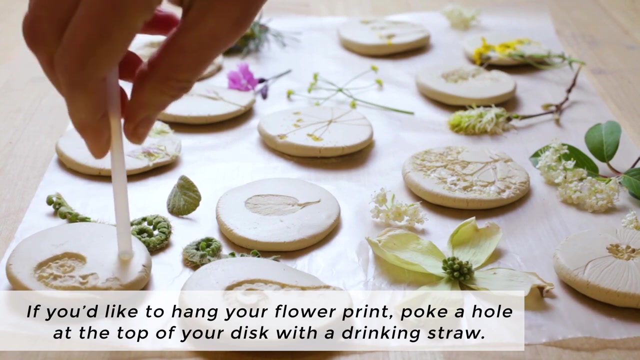 out and 96% of the air will go away. Carefully lift the clay disc, turn it over and peel away the flower or the leaf. If you'd like to hang your flower print, then poke a hole at the top of the disc with the drinking straw. 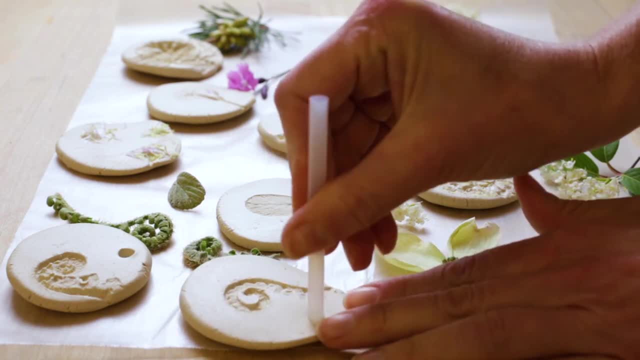 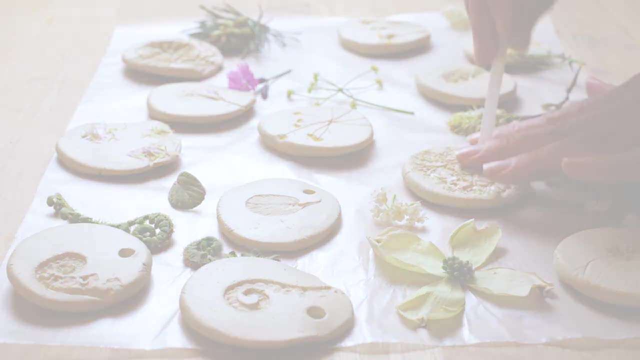 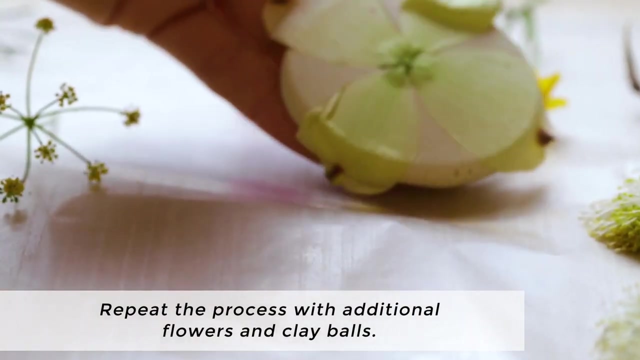 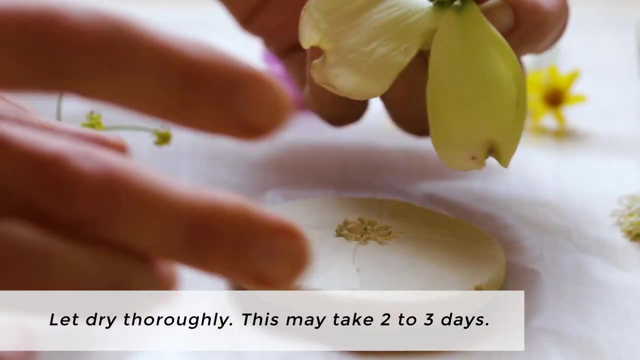 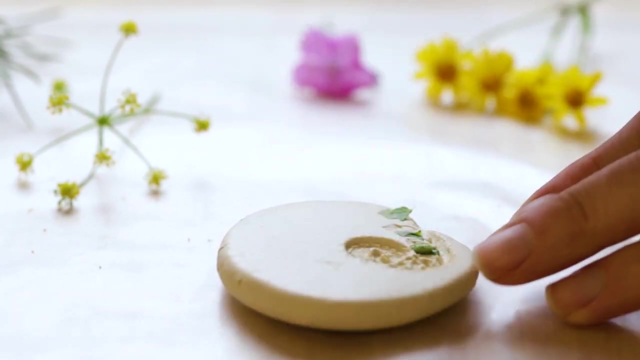 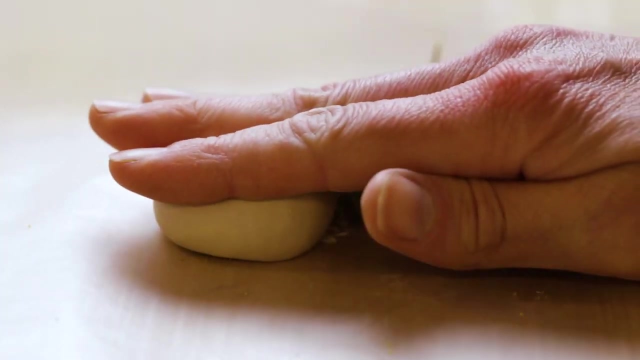 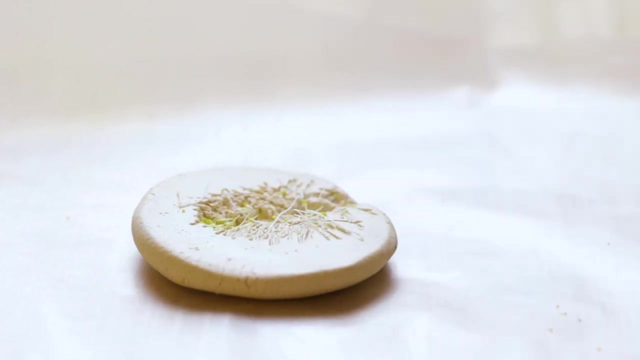 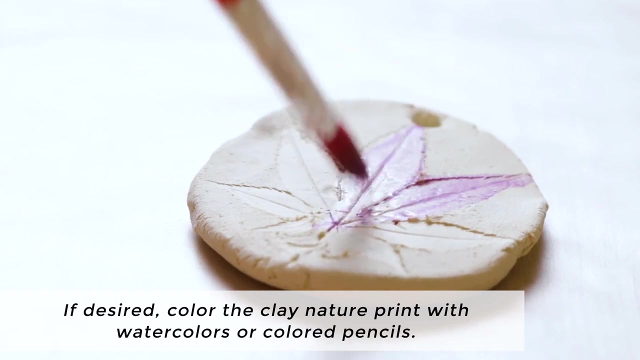 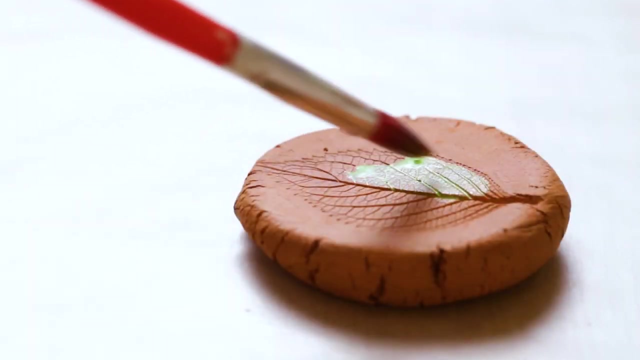 Repeat this process with additional flowers and leaves and clay balls And let your nature prints dry thoroughly. This may take two or three days And then, if you like, you can paint the clay leaf prints or flower prints with watercolors or color them with colored pencils. 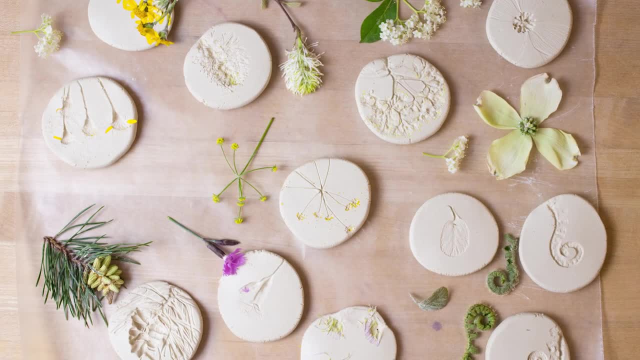 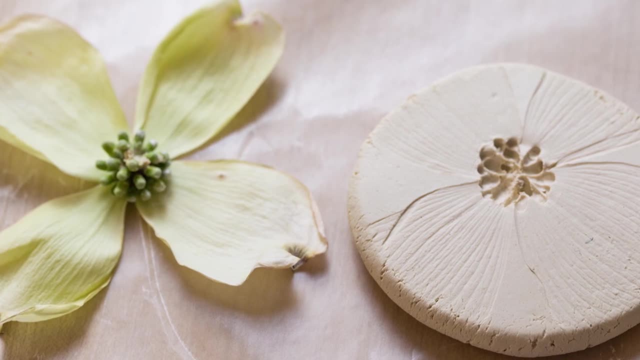 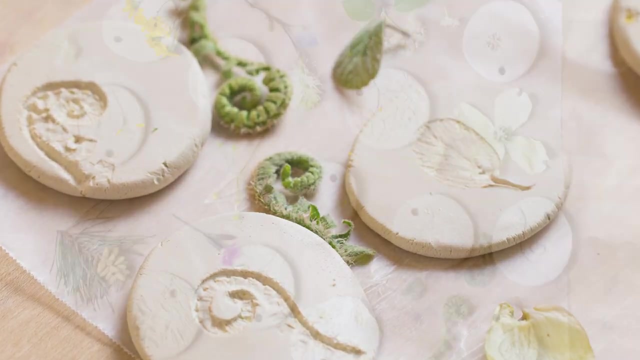 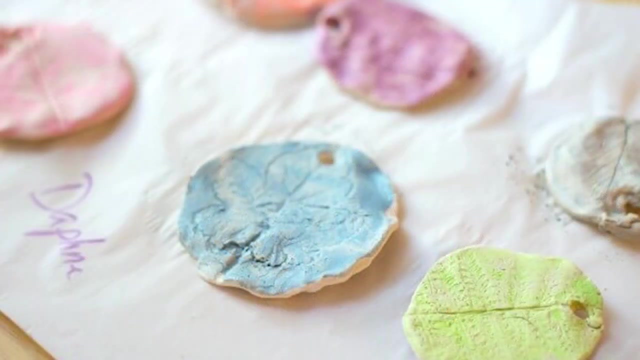 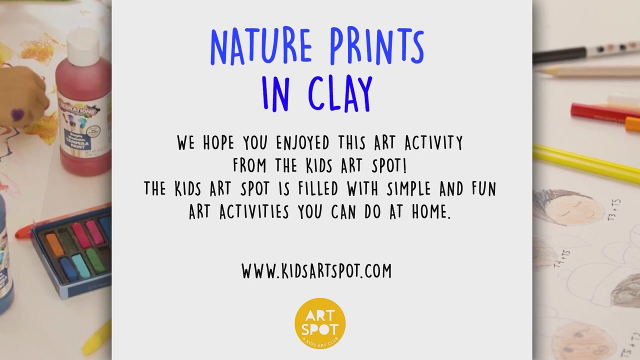 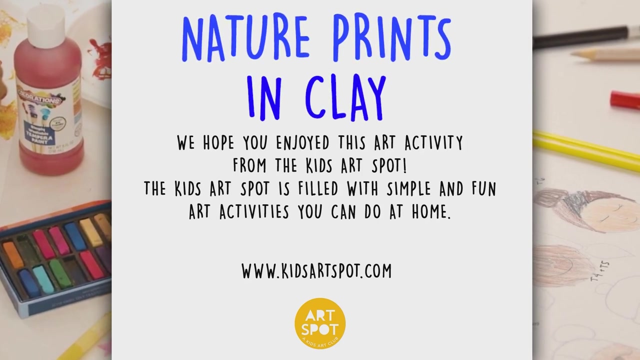 I hope you enjoyed this activity. If you liked this video, please share it with your friends on social media and leave a like if you enjoyed it. Thank you for watching and see you in the next video. Bye-bye.